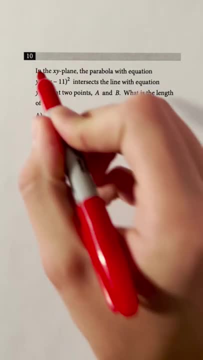 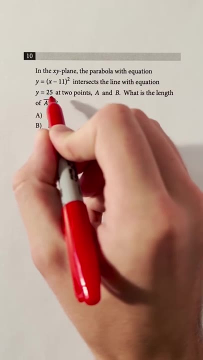 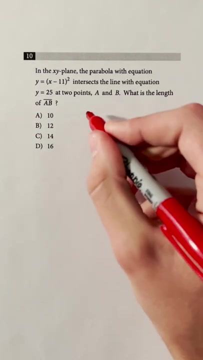 Make sure you can easily visualize graphs for the SAT. In the xy plane, the parabola with equation y equals x minus 11 squared intersects the line with equation y equals 25 at two points, a and b. What is the length of line segment a- b? To visualize what's going on, we have a parabola. 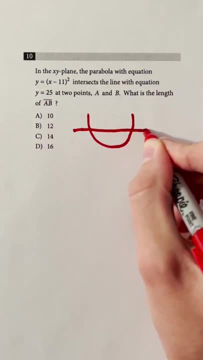 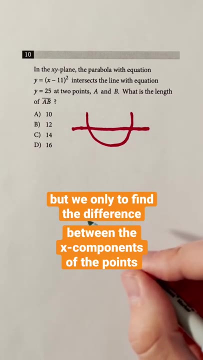 like this, and then a horizontal line cutting through at two points. We need to find the distance between the two intersection points, but we only need to find the difference between the x components of the points, Since the line between the two intersection points is horizontal. 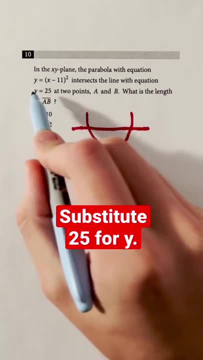 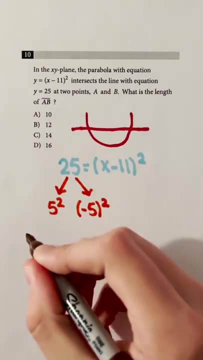 so the y components are not changing. so let's substitute 25 for y, and y equals x minus 11 squared. Notice that 25 is 5 squared or negative 5 squared. so x minus 11 equals 5 or negative 5.. 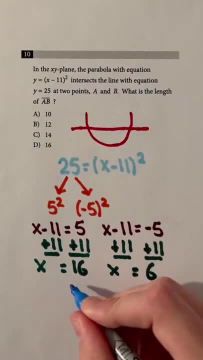 Thus x must equal 16 or 6.. The difference between 16 and 6 is 10,, so a is the correct answer. 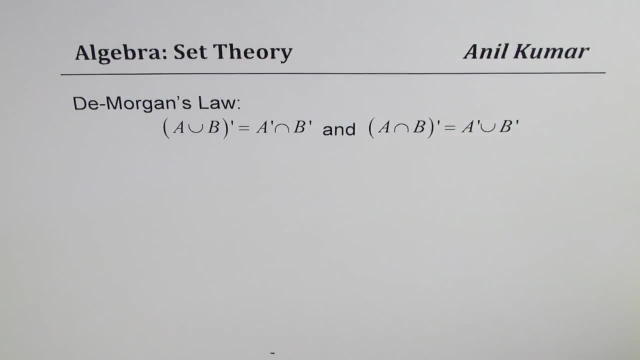 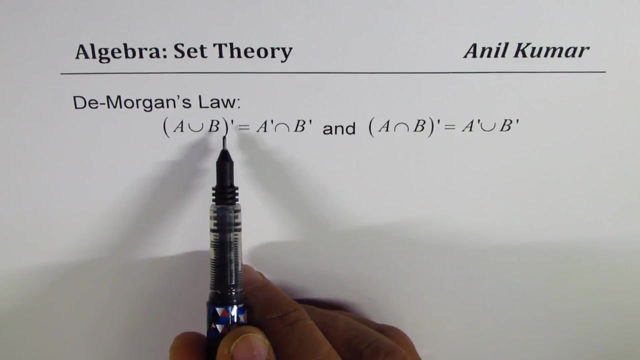 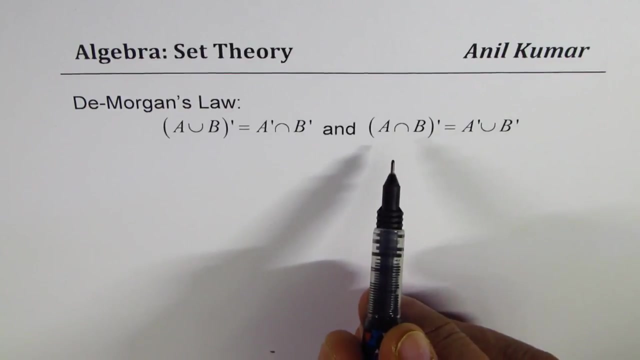 I'm Anil Kumar and in this video we'll talk about a proof for De Morgan's law. It's a very important law for set theory. It has two parts. The first one is that A union B complement is equal to intersection of complement of A and B, and the second part is that complement of intersection. 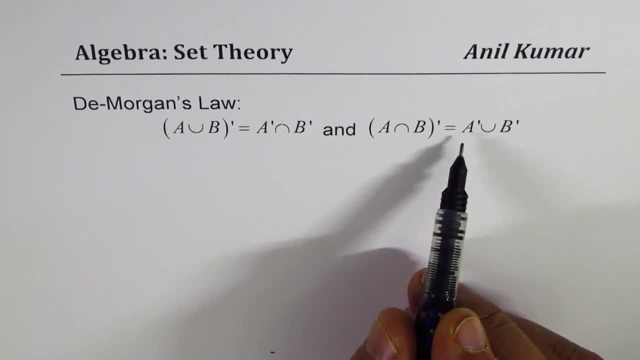 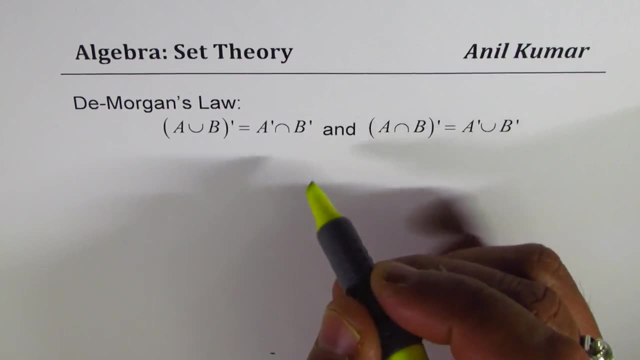 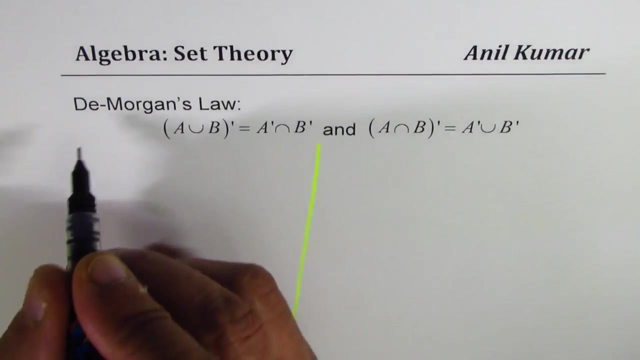 of A and B is equal to union of complements of A and B. We'll prove them algebraically right. So let's take the first one, which is complement of A union B. Let me call this as the first one. Now, to prove it, let us say that we have any x element which belongs to